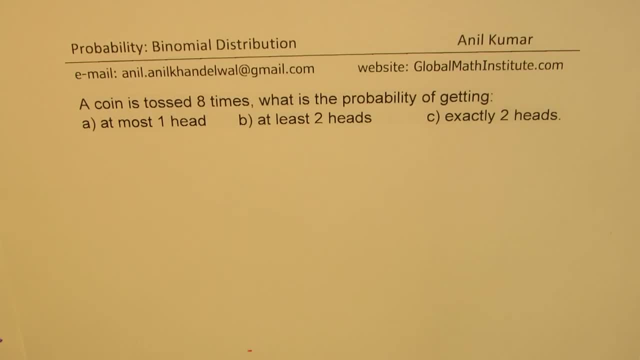 I'm Anil Kumar. Welcome to my YouTube channel and the website, Global Math Institute. Let me thank all my viewers and subscribers for participating actively and sharing good questions from all over the world. Here is a brilliant question from one of our subscriber, Mayhem. We'll see how to solve this question based on probability. The question here is: 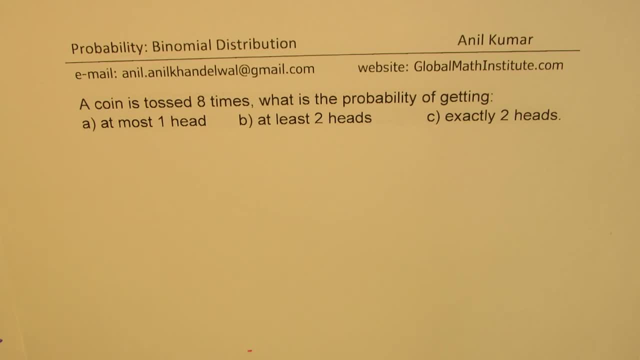 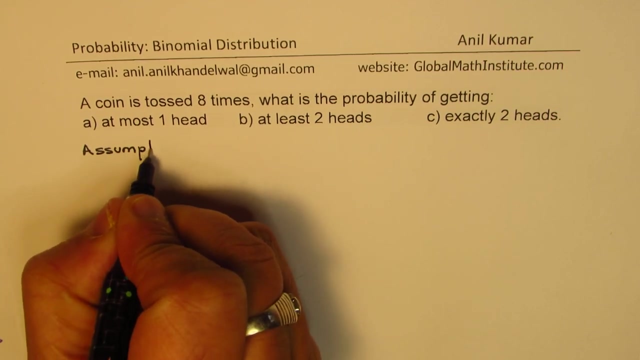 a coin is tossed eight times, What is the probability of getting at most one head, at least two heads, exactly two heads? A very important question indeed, So we'll assume few things here. So our assumption here is that we have a fair coin. right, So we have a fair coin. 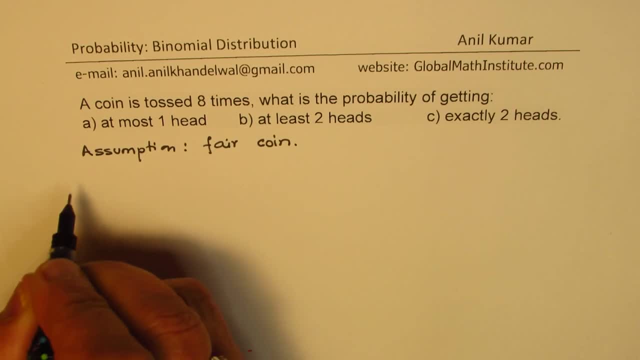 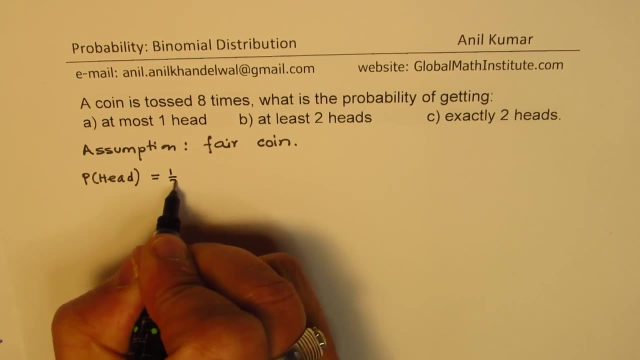 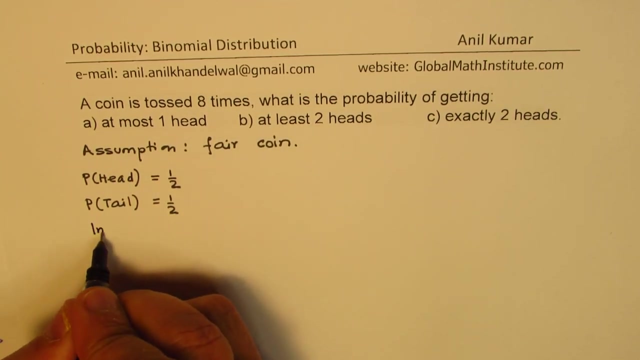 So that means the probability of getting a head is half and probability of not head- which is tail, in this case right- will also be half. We also realize that every event is independent event, So that means that the probability will not change. It will remain the same for every toss. 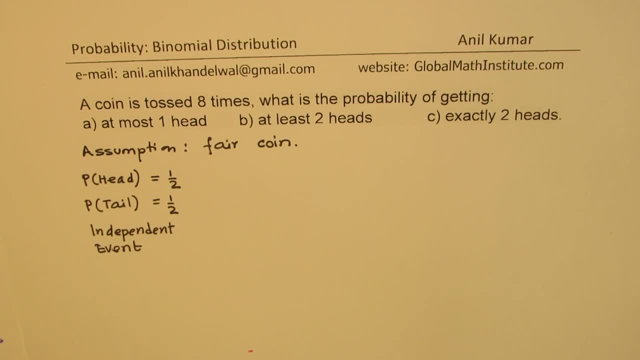 Perfect. So with these assumptions, we'll move forward. Now, some of you will also recall that this kind of probability is also referred to as a binomial distribution. So let's look at the binomial distribution. So this is a binomial distribution. 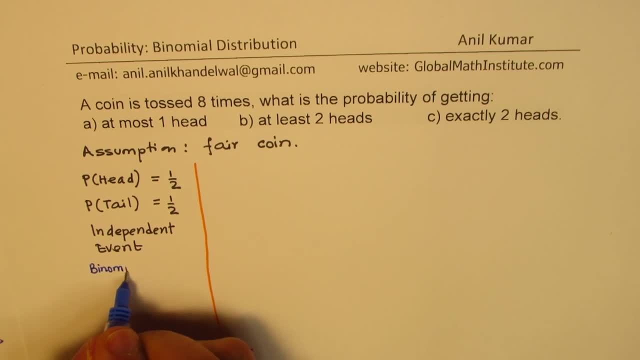 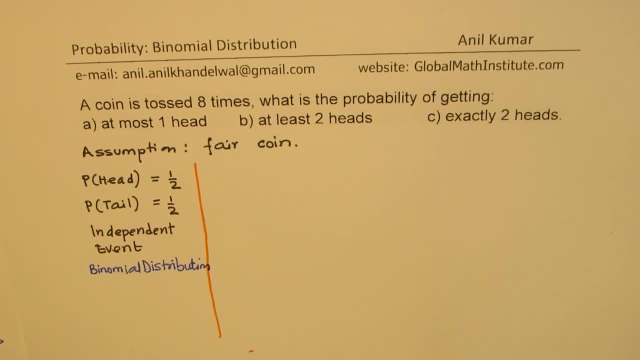 to answer this particular question right Now. we're talking about at most one head, at least two heads, exactly two heads. So we'll define our event as the event will be where the chances of getting heads right, So to get head. 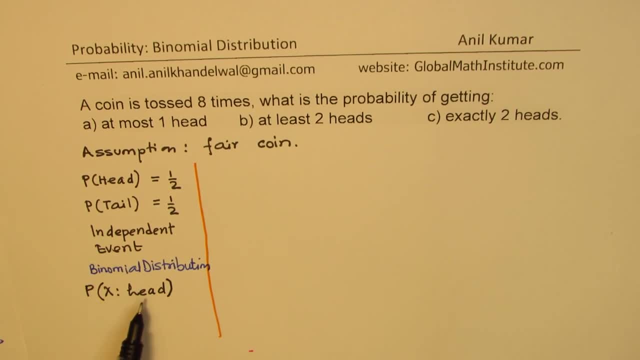 So the failure will be tails. but the success of an event is number of heads. So if we have eight times toss, then the number of heads could be one to eight, including zero, zero to eight. So there are nine possibilities, correct? 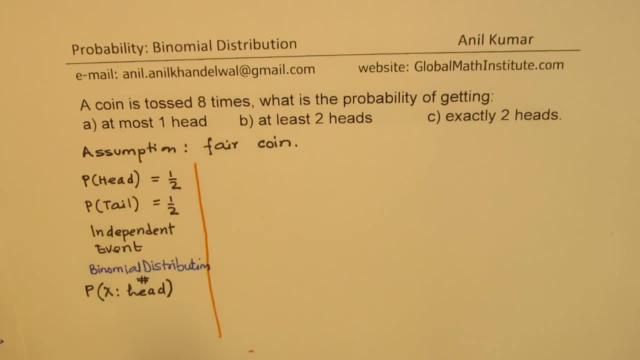 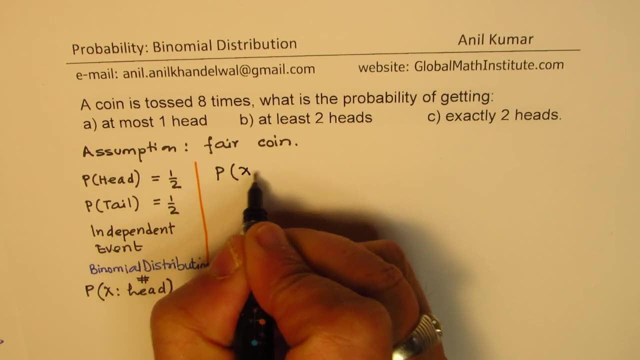 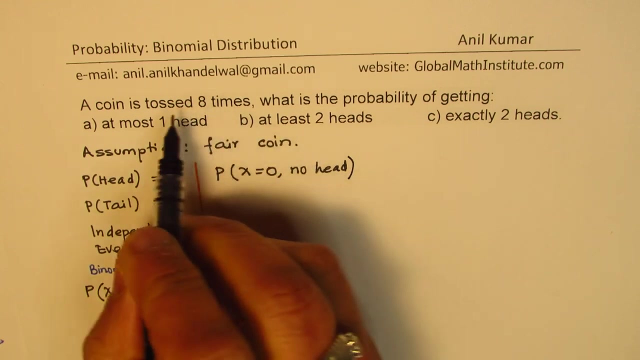 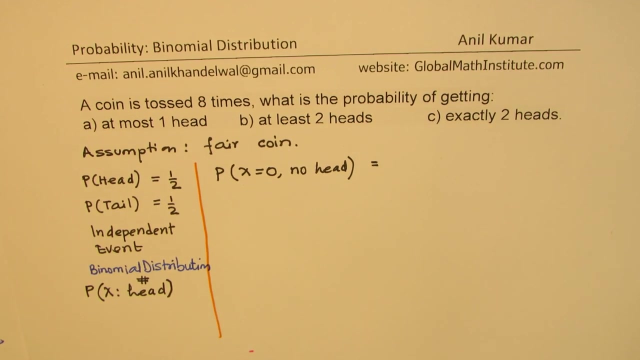 Now to answer these set of questions, let us begin by finding probability of x equals to zero. That means no head in eight tosses right. So that means no head means all the time when you toss you get a tail right. So we could write this as: 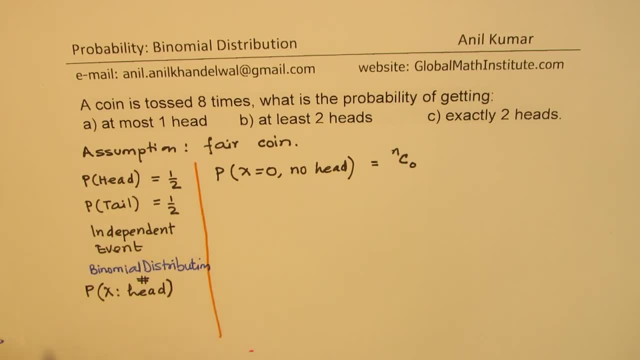 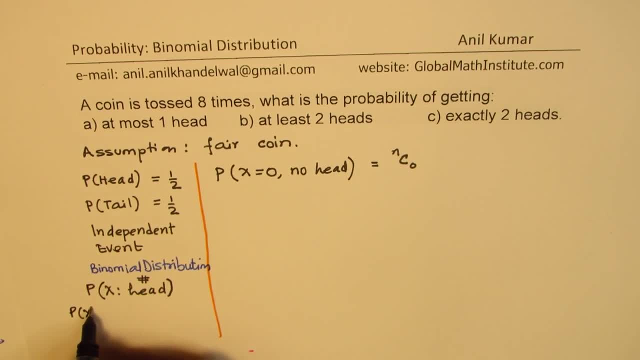 Nc0.. Nc0. Nc0.. When we're talking about the probability, then the probability can be written as Ncx success. let it be p, then the probability of p is whatever times x, times q, to the power of n minus x. 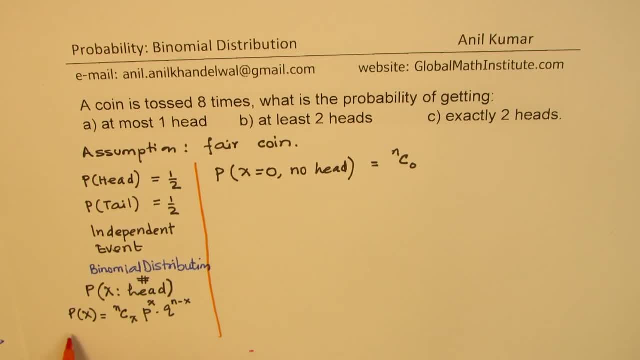 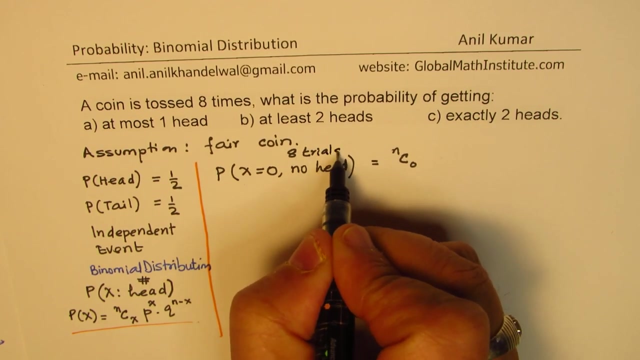 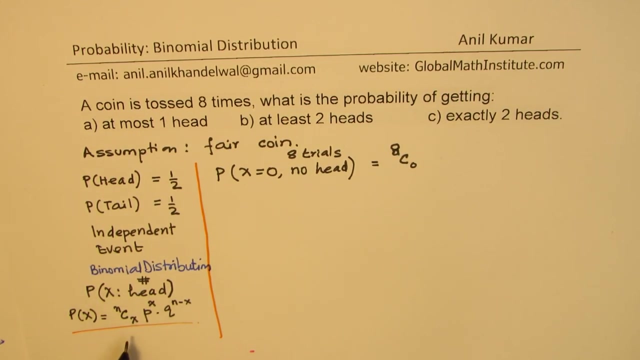 So that will be the general formula which will be used to solve this particular question. So when I'm saying no heads and we are saying no heads and we have eight trials, So we'll make this as eight. So there are eight trials, no heads. Probability of getting head is 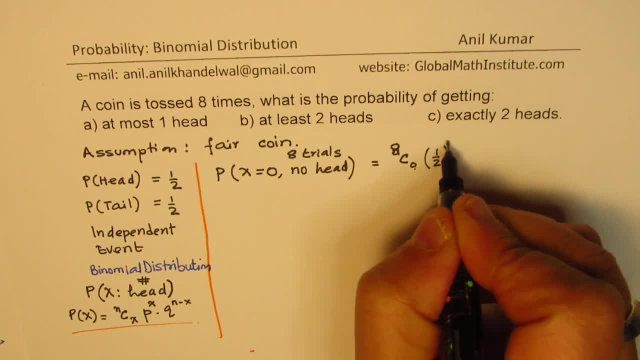 half, So well, half. and we get no head. and every time we get a failure, failure will be tail, and that will be eight tails. So now, if we have an easy question, that's going to be a little bit easier. 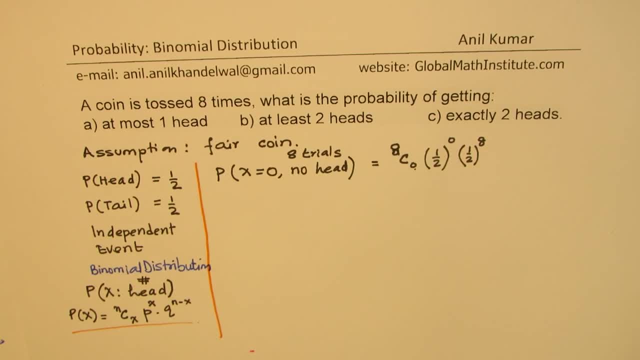 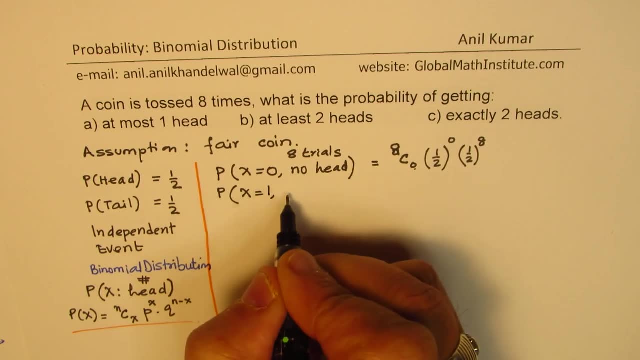 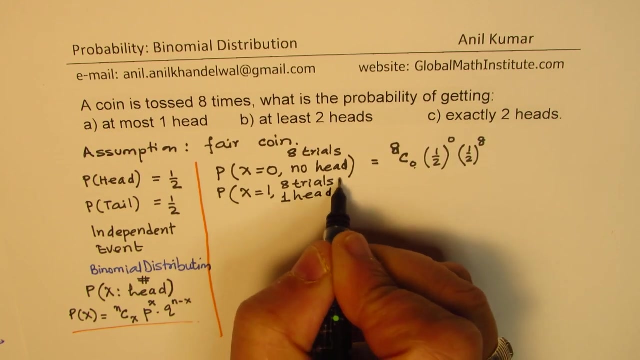 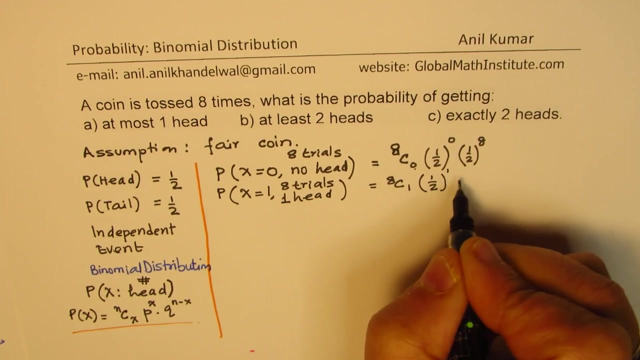 times. so that is the probability of no heads. perfect. let's find the probability when our random variable x is equal to 1. that means 8 trials and we have one head right. so in that case it will be 8 c, 1, half probability of head and this is half. 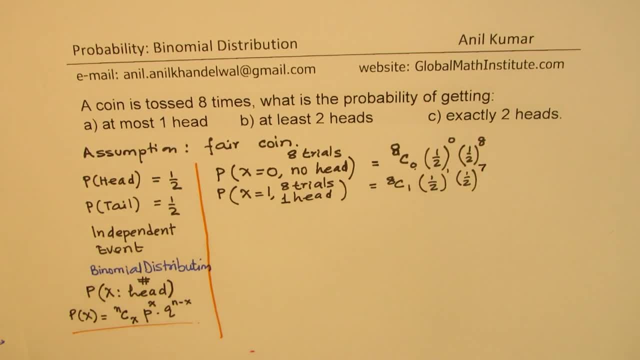 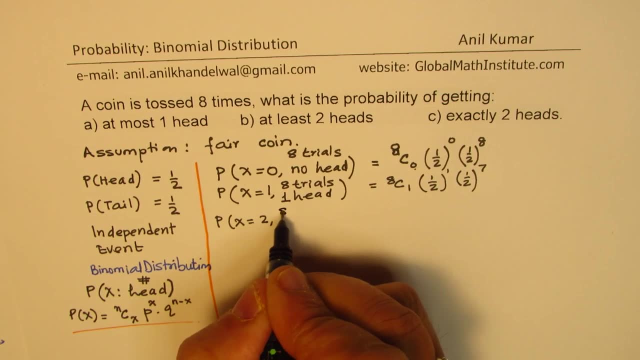 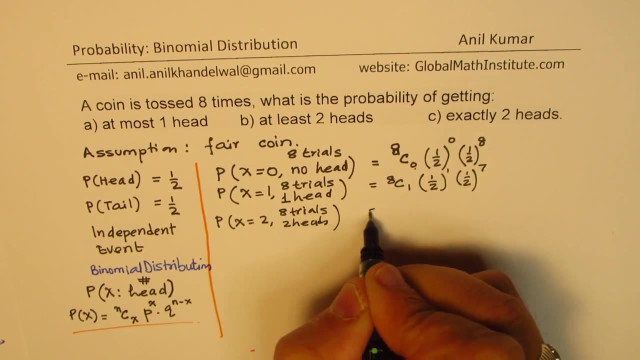 probability of tail will be 8 minus 1, which is 7. let's also see what is the probability of getting two heads. so 8 trials two heads. so out of 8 we have two heads. they could be in any position. right, that is what we mean when we 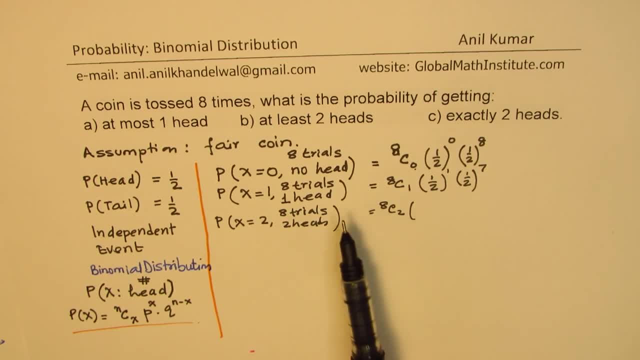 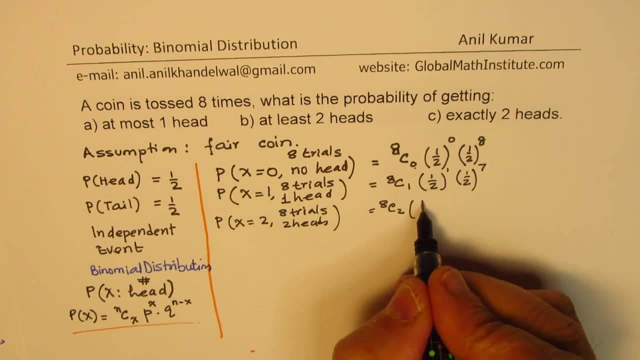 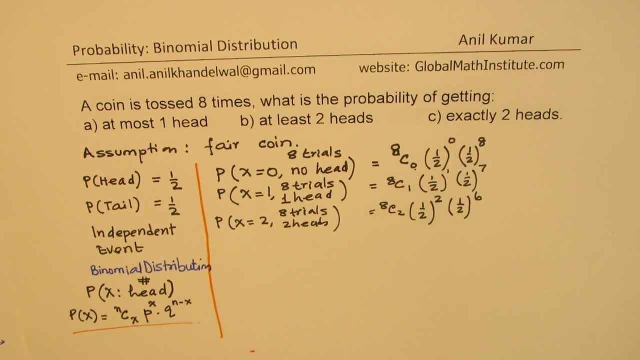 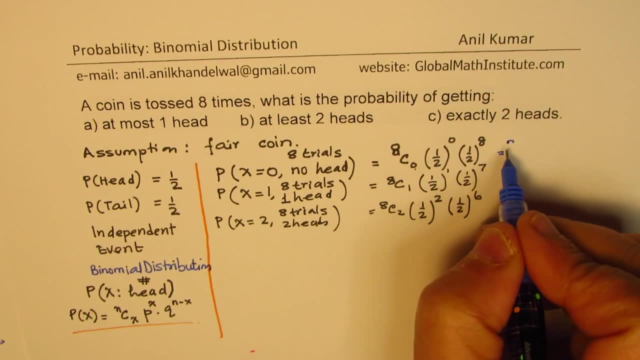 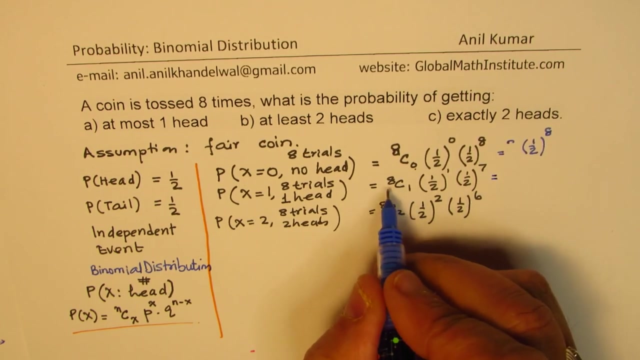 tail correct. so, in a way, what you see from here very clearly, that these probabilities are 8 c 0. okay, let's write: 8 c 0 is 1, right, so? so we can write this as half to the power of 8. right, that is 1. so we get half to the power of 8. now, in this case, what we get? 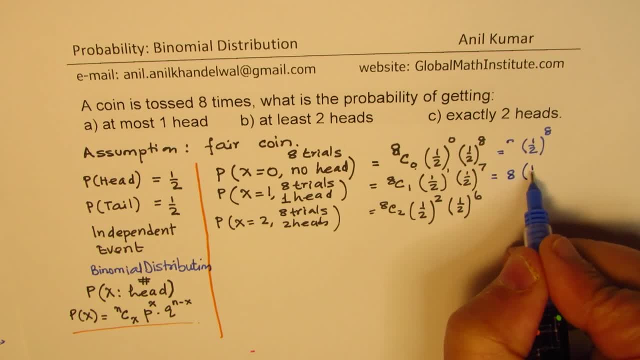 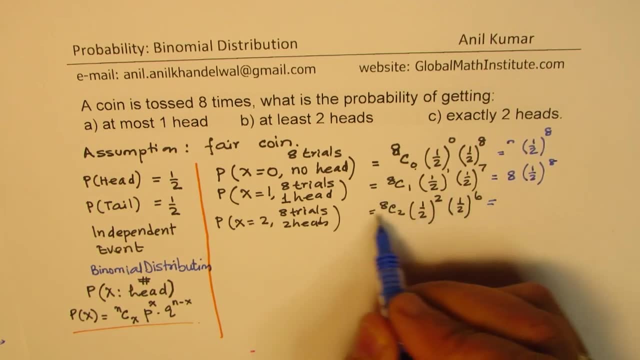 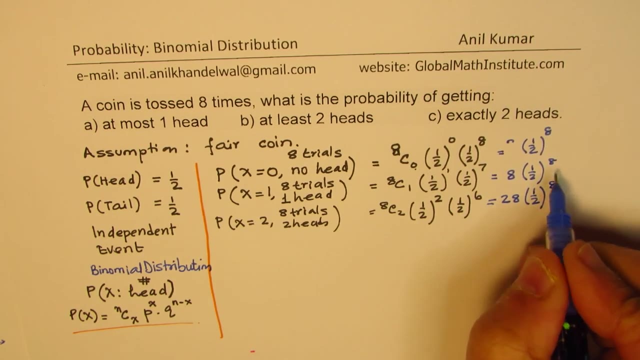 is 8 c 1 is 8 times right. half to the power of 8, again. and 8 c 2 will be 56 divided by 2, which is 28, half to the power of 8, again right. so those are the probabilities for exactly no head, one head or two heads. 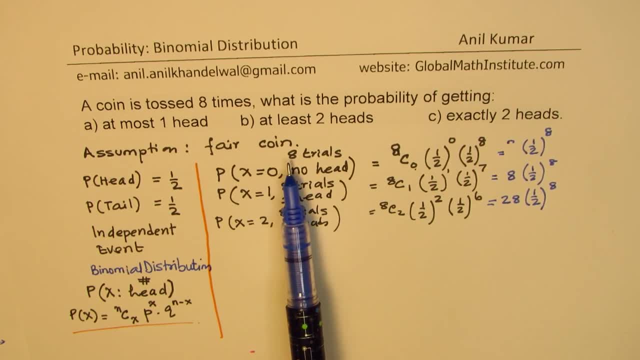 when you are throwing or tossing the coin, eight times, a fair coin is being taken. now let us answer the question. part a, part a, is at most one heads when say so, property of getting at most one, at most one head. I am mixing the nomenclature since I exactly don't know how much are you familiar with the. 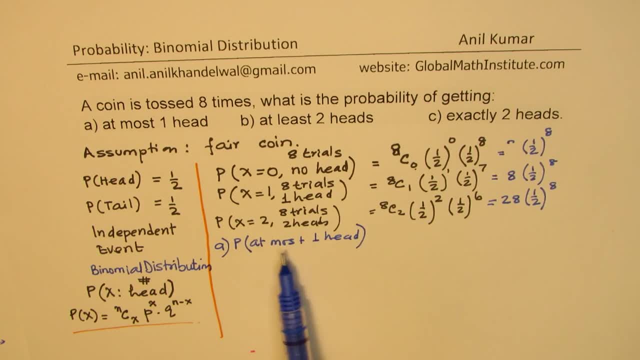 binomial distribution, so I'm trying to keep it simple, right, so I'm writing it in plain English. so, at most, one head means what? either you get zero heads or you get one head. so that means 0 or 1, right, so it is. it is the probability. 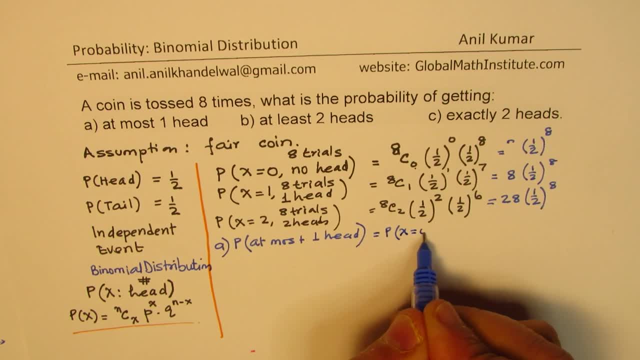 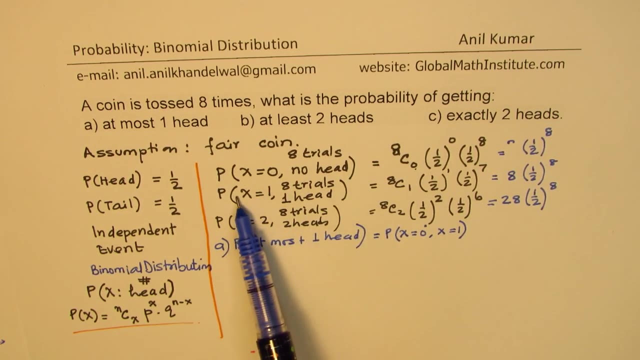 when the value of X is 0 right, or X is equal to 1, so at most one. okay, so that means we'll add the first two right, so no heads and the probability of getting one head. so we are going to add the first two. so what? 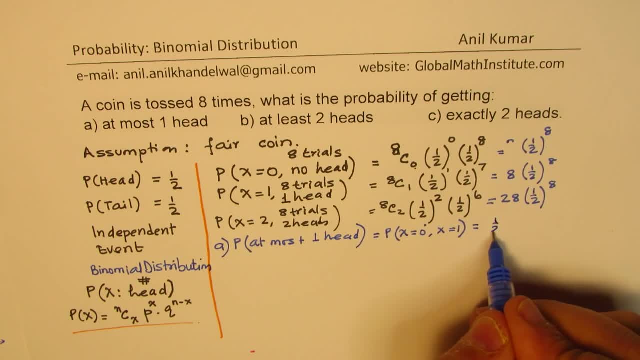 we get here is half to the power of 8 plus 8 times half to the power of 8. is that clear? so that is going to be the answer of part a right. so that is 9. 8 plus 1 is 9, and 8 is half to the power, is 256. so we get 9. 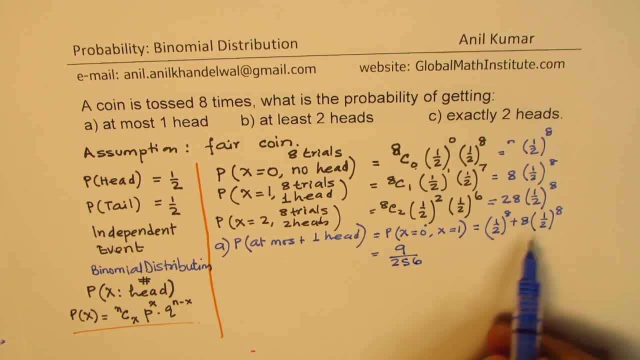 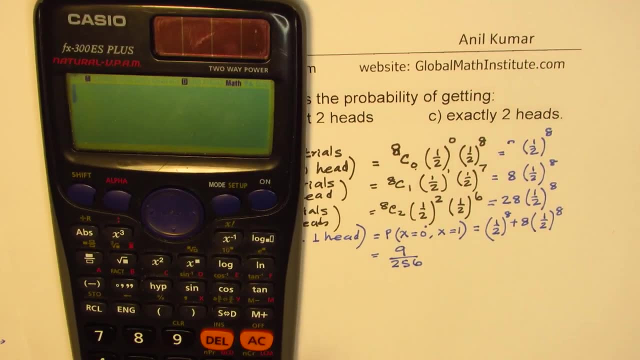 over 256. is that clear, right? so that will be our answer. you could use your calculator also. so basically we have, we can say 0.5 to the power of 8. half is point 5, which is 1 over 2 plus 1, which you can also. сделал this problem to the. 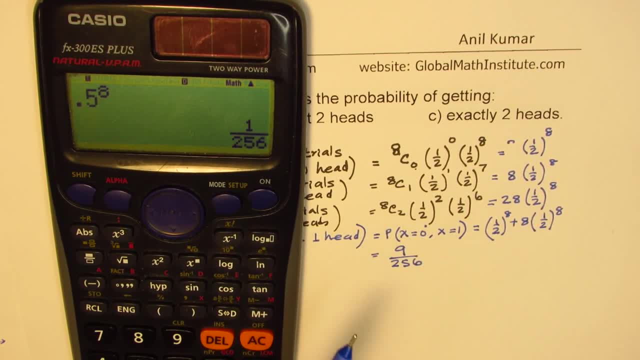 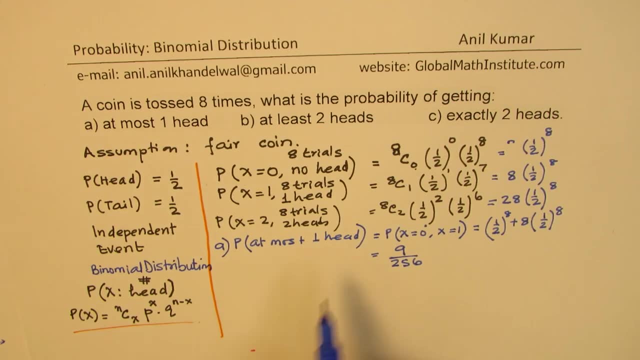 power of 8, half power over the power 256, and 1 plus 8 is 9, right? so times 9, so we get 9 over 256 as answer for first part. now let's look into part b. part b is at least two heads. at least two heads means 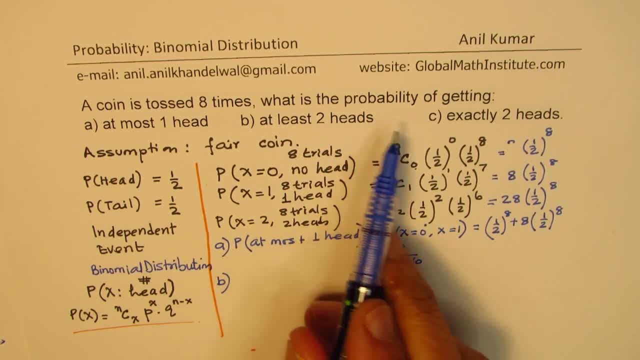 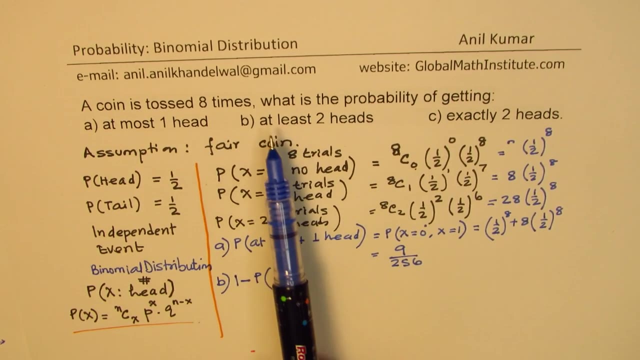 you get 2, 3, 4, 5, 6 and so on. so that means we are looking for 1, minus probability of getting what we'll not look into- probability of getting tails right. so so when you say at least two heads, that means we are not considering the case where we have zero heads or we have one head. 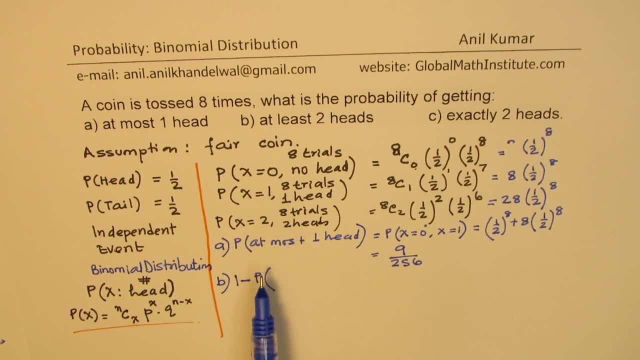 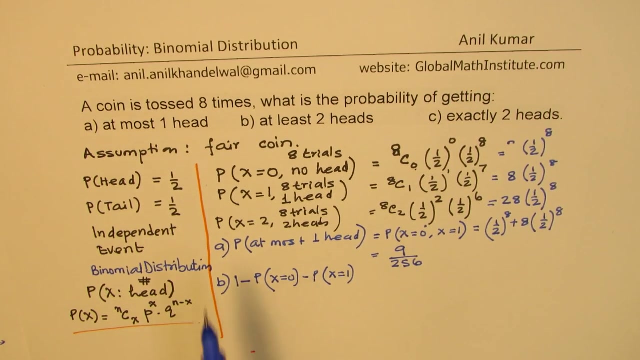 correct. so probability of- so let me write- minus probability of getting no heads when x equals to 0, minus probability when x equals to 0. is equal to 1, correct. so those probabilities we have to take away to get part B, at least two heads. so we get either two heads or three heads. four: 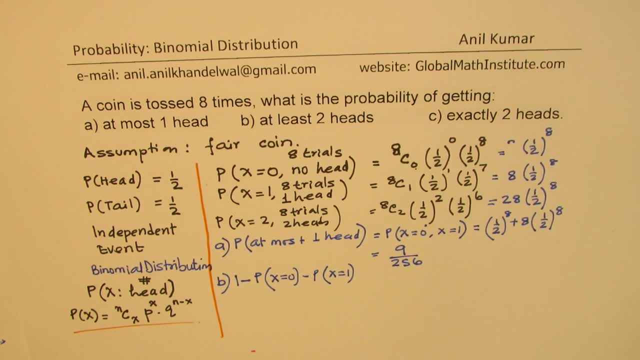 heads- five, six, seven or eight heads- correct, but we will exclude the probability of getting one head and no heads. so we'll exclude this part. great, so this could be written as 1 minus. we already find this, which is 9 over 256. is that clear to you? so that becomes the probability of getting at least two. 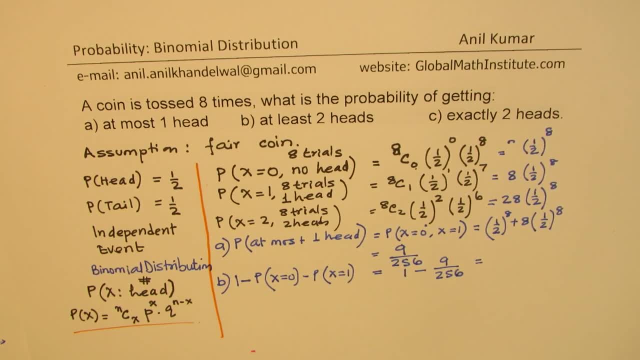 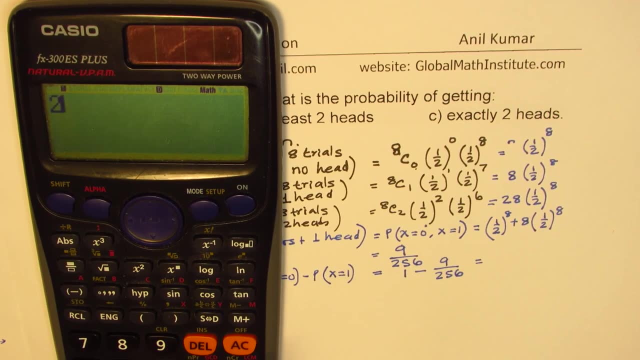 heads. so 1 minus this probability, and we can use the calculator once again and figure this out. or 256 minus 9 over 256, correct? so 256 minus 9 different divided by 256. so we get this answer as 247 over 256. is that clear to you? perfect? 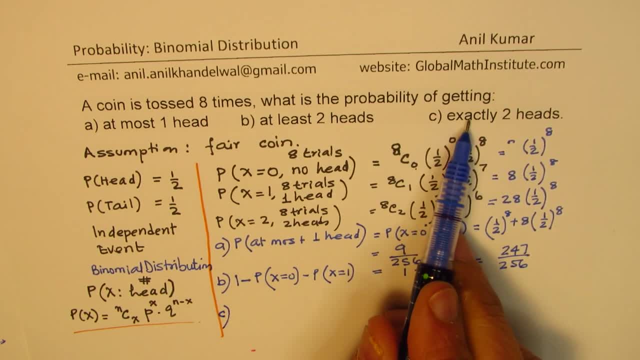 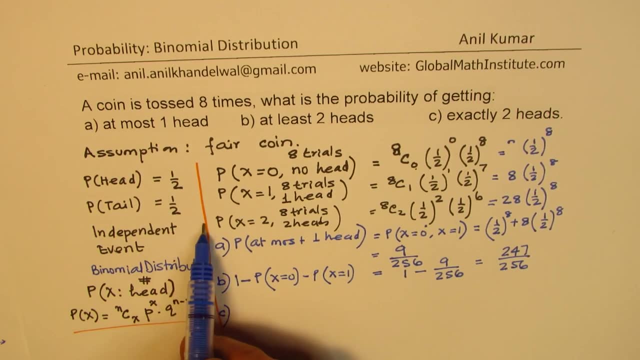 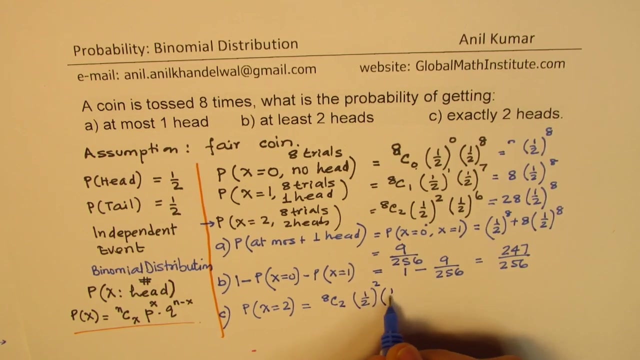 now part C is exactly two heads. so when we are looking for probability of exactly two heads, means that option correct. so probability for the value of heads when two is 8c, C to half to the power of 2 and half to the power of six right, so which is 28. 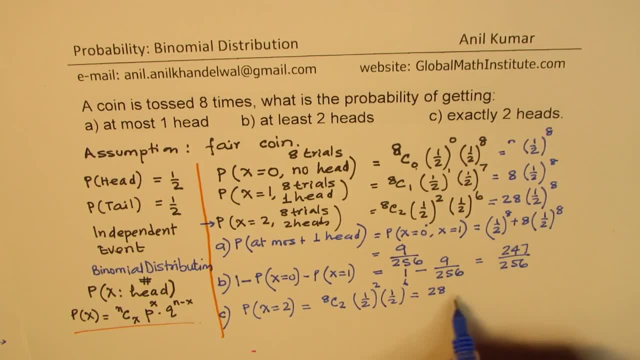 times 1 over 8, 1 over 2 to the power of 8, which is 28 over 256. okay, so you could simplify this. we can divide by 4, so we get 7 over. dividing by 4, 4 times 6 is 24- 64, right, so get 7 over 64 as our answer. so for 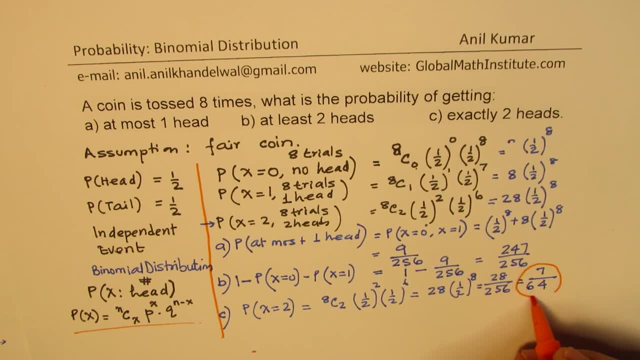 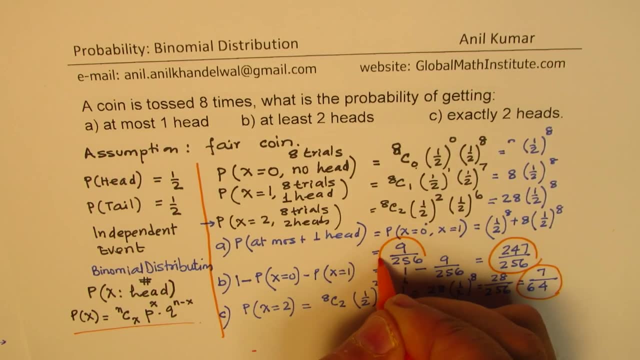 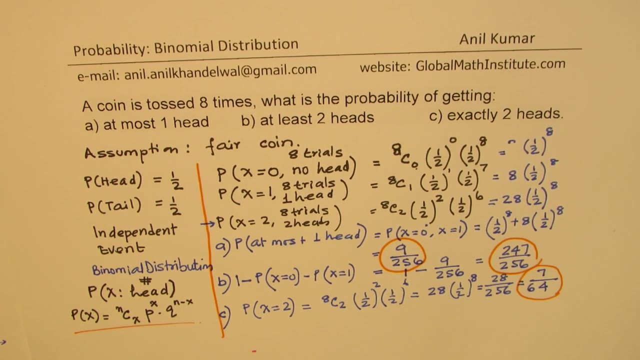 these three events, the answers will be 7 over 64 for the last one. the second last one is 247 over 256 and the first one is 9 over 256. perfect, so I hope you understand- and with this you also understand the terms- at most one head.